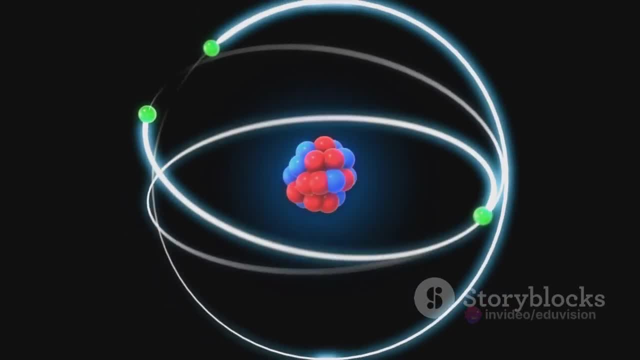 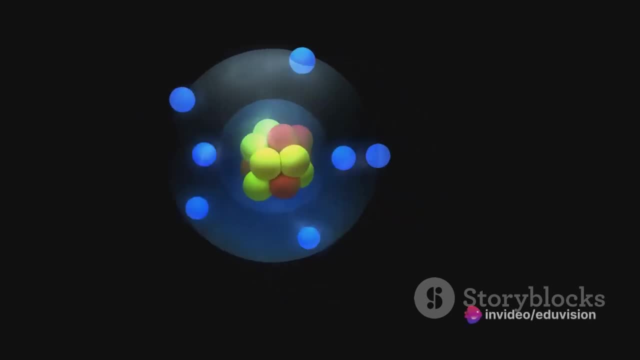 and your fridge cold. Next, we delve into the subatomic world with the strong nuclear force, the glue that binds protons and neutrons in an atomic nucleus, keeping atoms together and making our existence possible. Finally, we meet the weak nuclear force, the shy character. 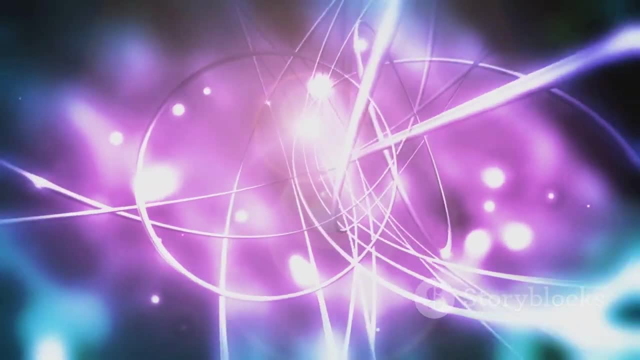 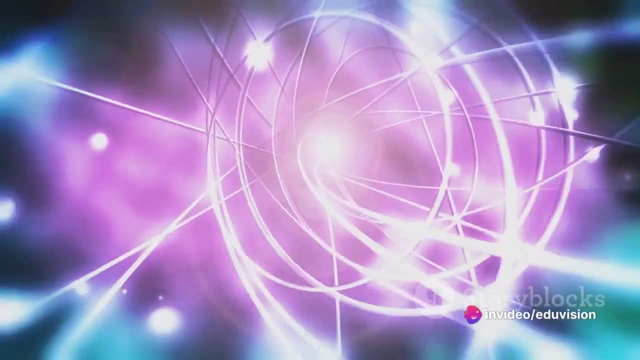 responsible for radioactive decay and nuclear fission powering our sun and stars. Now imagine a theory that unifies these forces into one. That's where our story begins. In the wake of the 20th century, physicists began to dream of a theory that could unify. 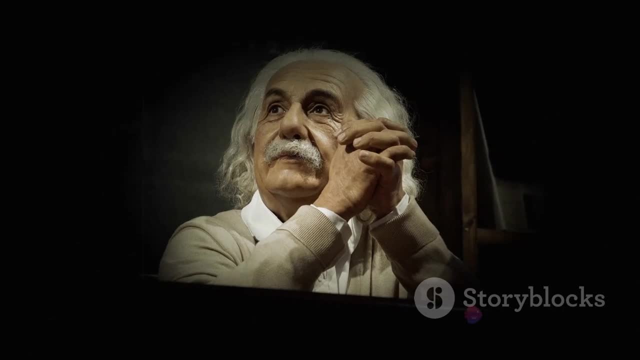 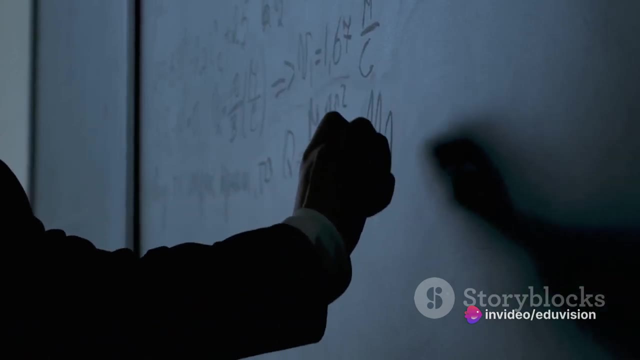 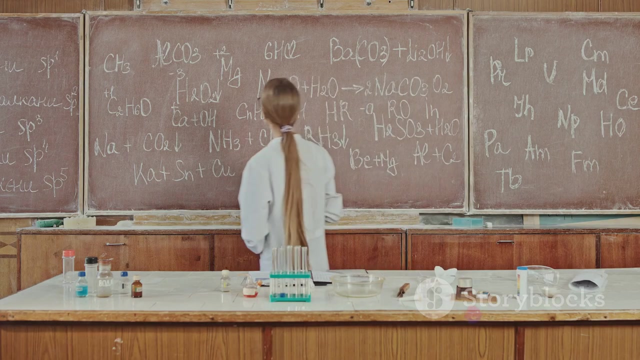 the fundamental forces. The seeds of this aspiration were sown by the pioneers of quantum mechanics and relativity. It was their groundbreaking work that laid the foundation for what would eventually become the Grand Unified Theory, or GUT. The journey started with a focus on unifying two of the four fundamental forces of nature. 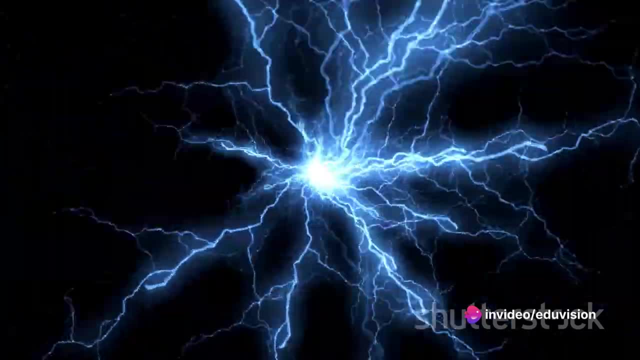 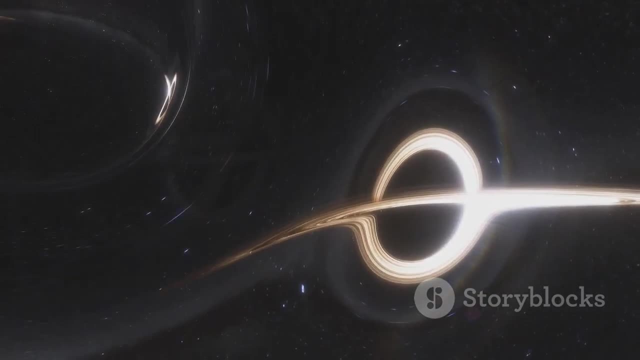 Electromagnetism and the weak nuclear force. These forces, vastly different in strength and reach, were considered separate entities. However, in the mid-20th century, theorists proposed that, at high enough energies, these forces could be seen as two aspects of a single electro-weak. 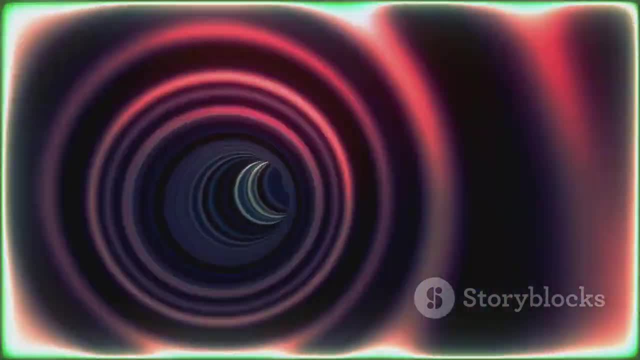 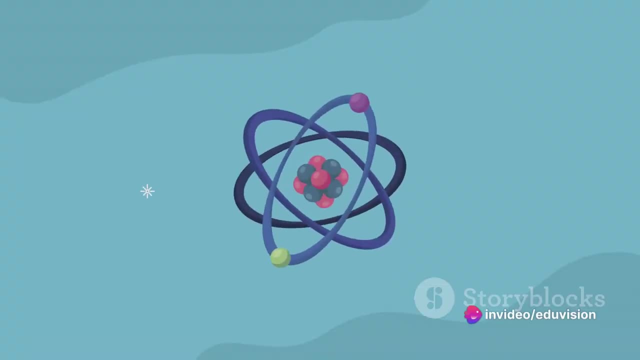 force. This groundbreaking idea was the first step towards the birth of GUT. The next challenge was to incorporate the strong nuclear force into this unified framework. The strong nuclear force as, as its name suggests, is the strongest of all forces at a subatomic level, It holds the protons. 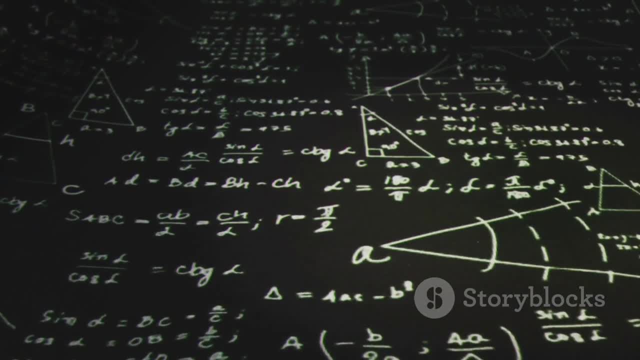 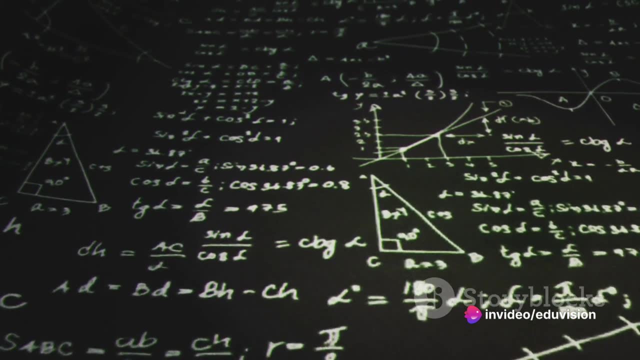 and neutrons within an atomic nucleus together. Physicists hypothesized that at even higher energies this strong force could also become part of the electroweak force, giving birth to the grand unified theory. This was a bold and ambitious idea. It suggested that at the very 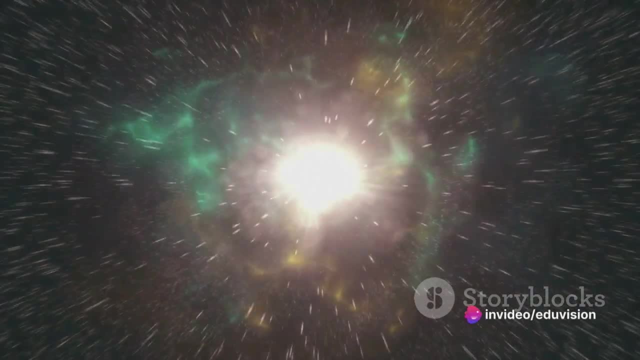 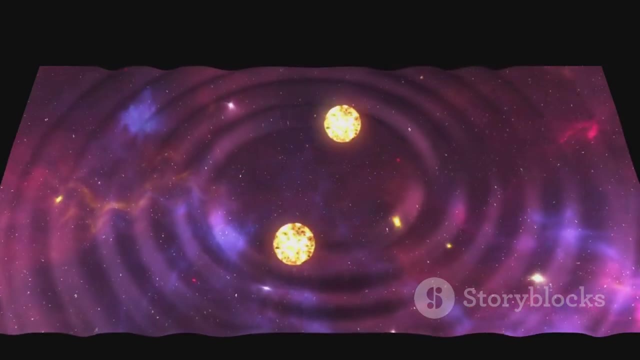 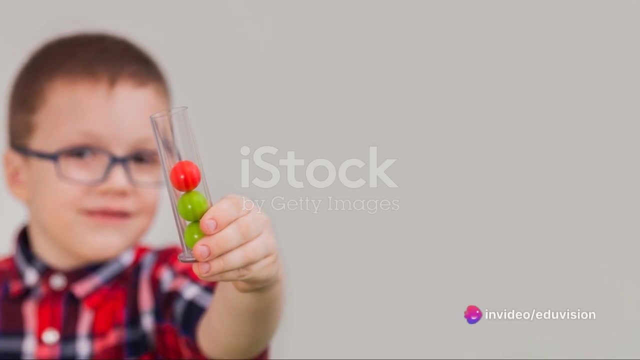 beginning of the universe. in the intense heat of the Big Bang, all forces were unified into one. As the universe cooled and expanded, these forces broke into the separate entities we see today. However, the path to this unification was not straightforward. Physicists had to reconcile: 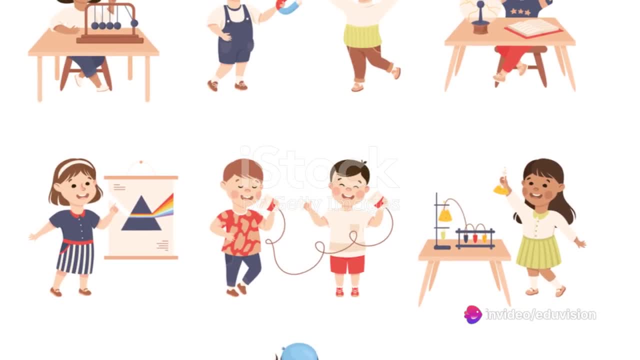 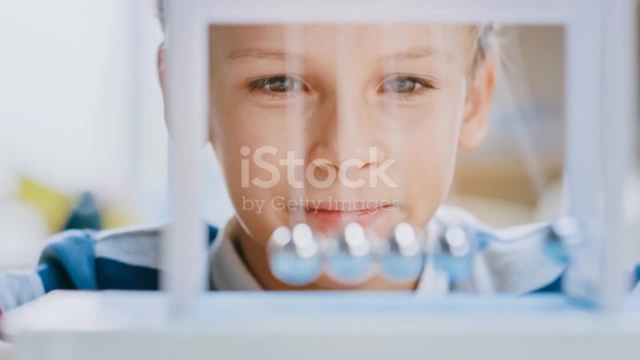 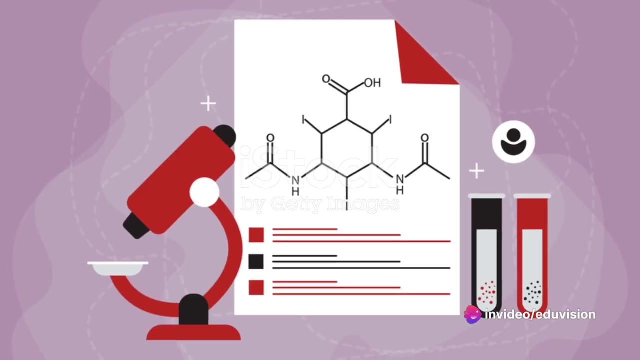 the discrepancies between quantum mechanics, which explained the world of the very small, and general relativity, which described the universe at large scales. This proved to be a complex and arduous task, and the journey towards the grand unified theory was filled with challenges and setbacks, While the idea was revolutionary. 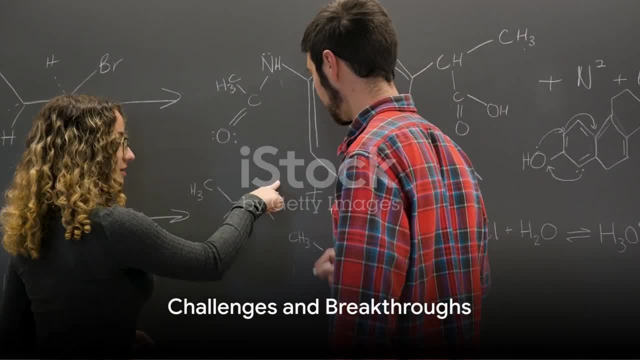 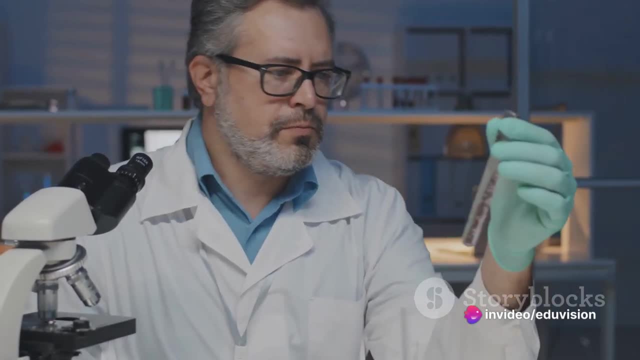 getting there was not a smooth journey. The path to unifying the fundamental forces was fraught with challenges. This journey, like many great scientific quests, was marked by its fair share of obstacles and setbacks, One of the most significant challenges in developing the grand 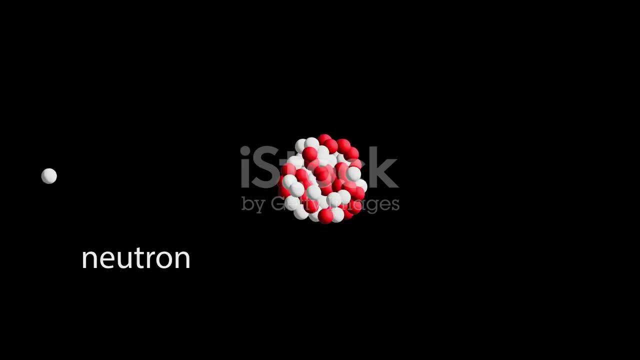 unified theory, or GUT, was the disparity between the predicted and observed proton decay. The GUT proposes that at very high energies the three forces electromagnetic, weak and strong merge into one single force. The GUT proposes that at very high energies the three forces electromagnetic, 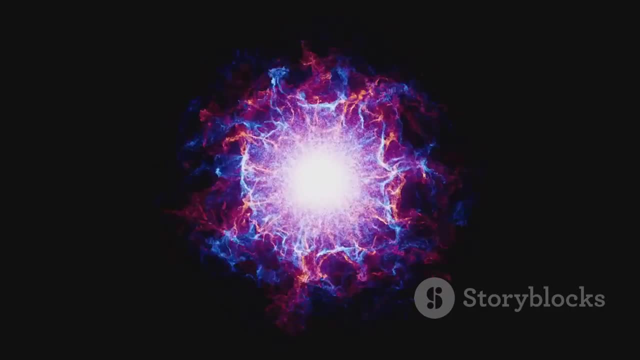 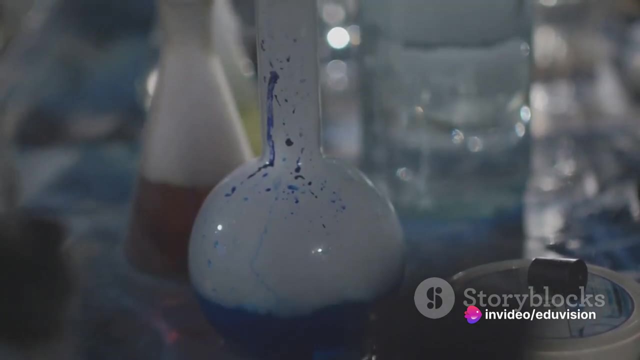 weak and strong merge into one single force. This implies that protons which are considered virtually stable within the standard model should decay over time. However, the predicted rate of this decay was much faster than what we've observed in reality, a discrepancy that posed 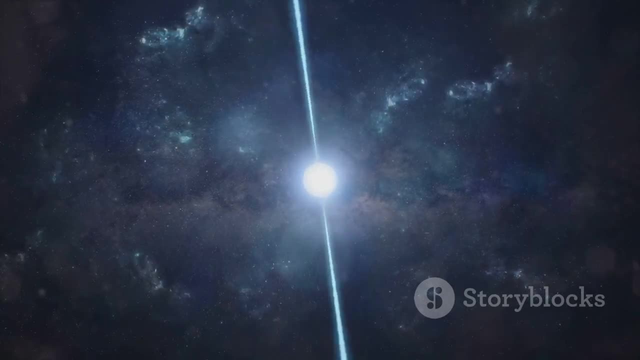 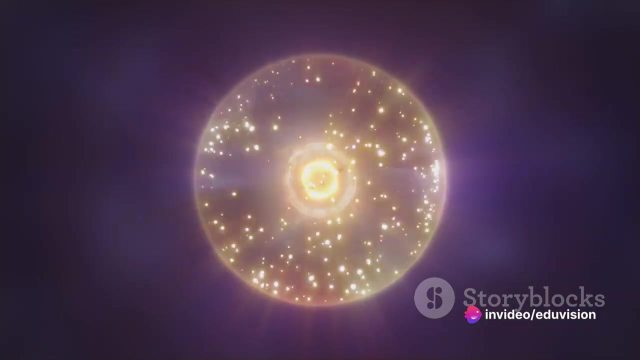 a significant roadblock in the acceptance of the theory. But science, as we know, is an ongoing process and breakthroughs often come when we least expect them. The introduction of supersymmetry, or SUSY, was one such breakthrough. SUSY suggests that each particle has a superpartner with. 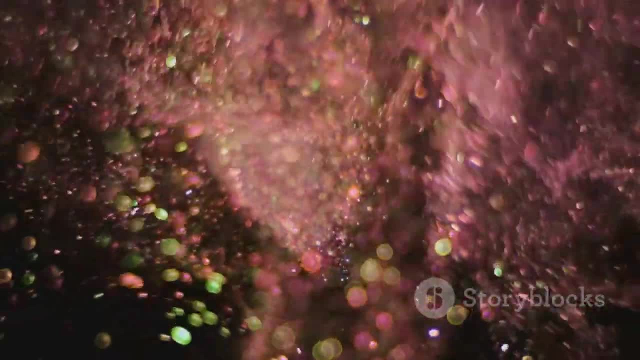 different superpartners. The superpartners are the superpartners of the superpartners. The superpartners spin, helping to resolve the proton decay issue by predicting a much slower decay rate, more in line with observations. Another major breakthrough was the discovery of the elusive. 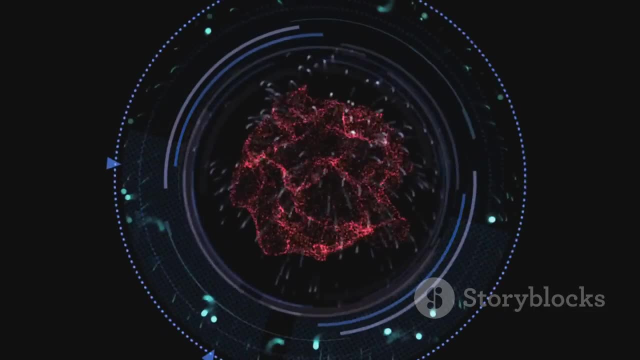 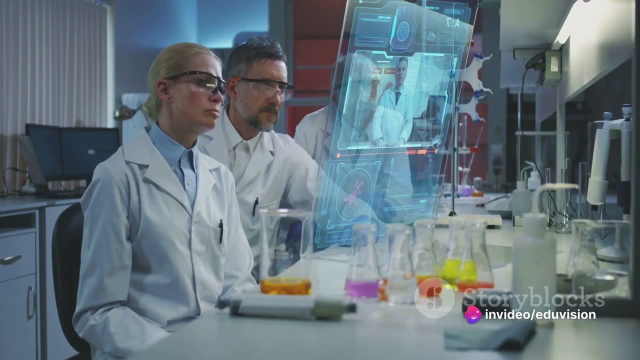 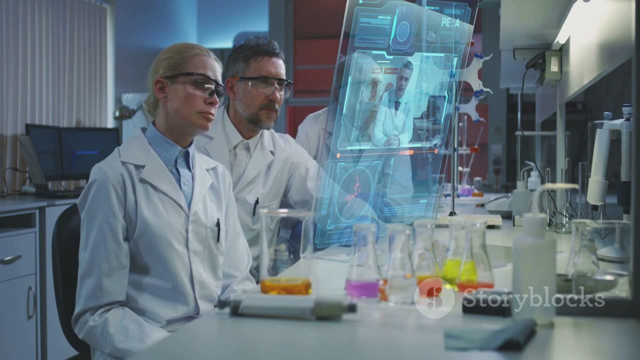 Higgs-Boson in 2012.. This particle, which gives other particles their mass, was the missing piece in the standard model of particle physics. Its discovery not only bolstered the credibility of the standard model, but also provided a significant boost to the concept of the grand unified theory. 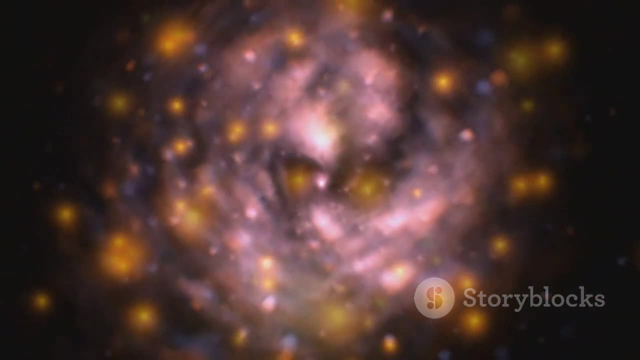 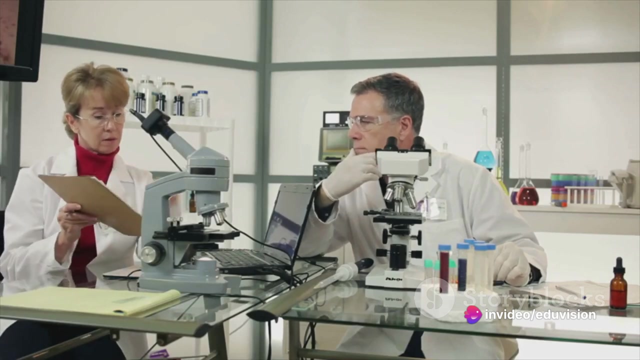 These breakthroughs, among others, have helped. the GUT proposes that at very high energies the universe is a fundamental force. They have opened up new avenues of research, sparked fresh debates and reignited the quest for a theory that can reconcile the quantum world with the cosmos. 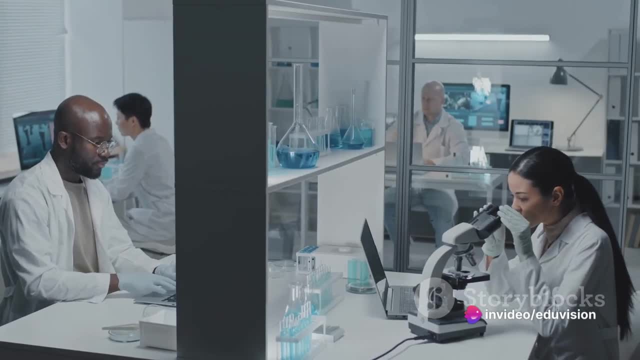 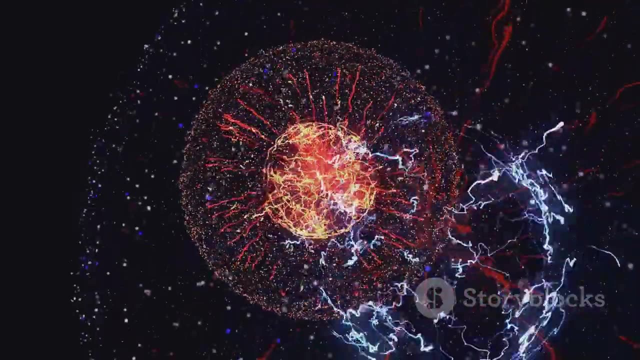 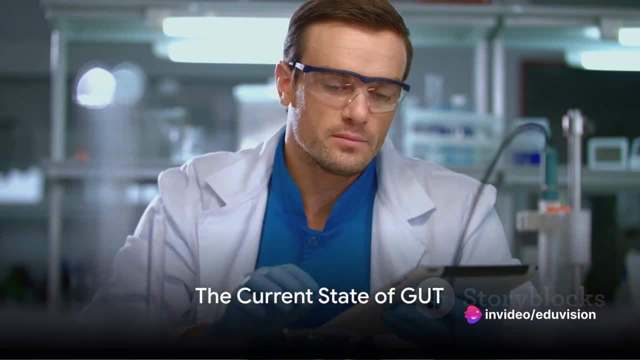 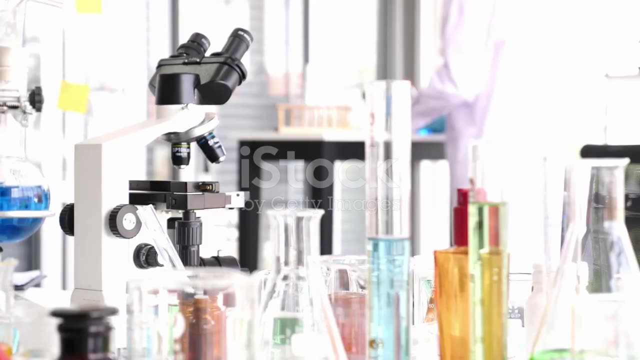 And with every step we take we inch closer to uncovering the secrets of our universe. So where are we now in the quest to unify the fundamental forces? Currently, the grand unified theory is in an exciting state of development. New FUCKING reality hasore Creatures made a statement about what would change. 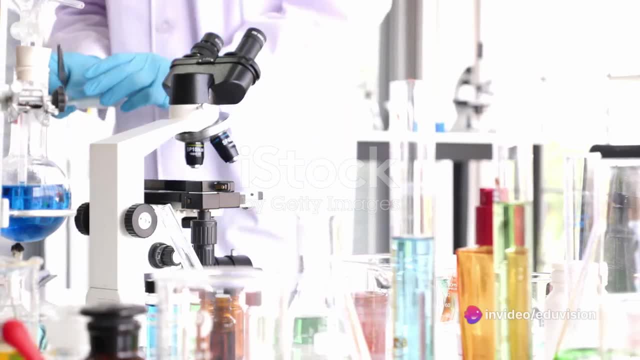 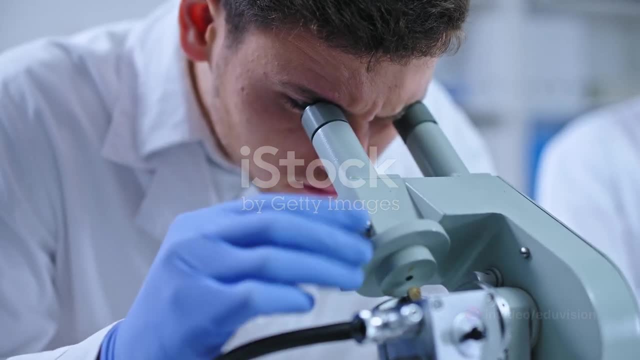 This is a drama growing in the era of круг agrade to predict the worlds overruling of a million years after the creation of the specific dahaan agriculture. Recent advancements have shown promise, sparking a renewed sense of hope within the scientific community. 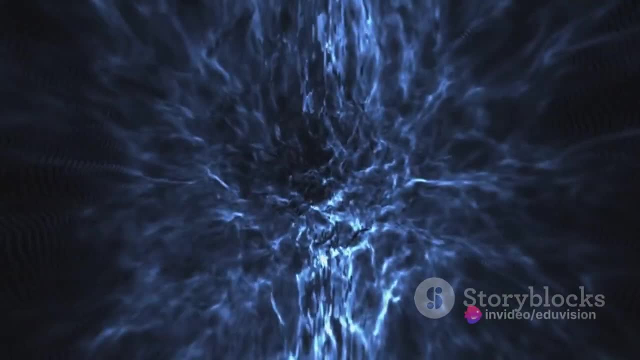 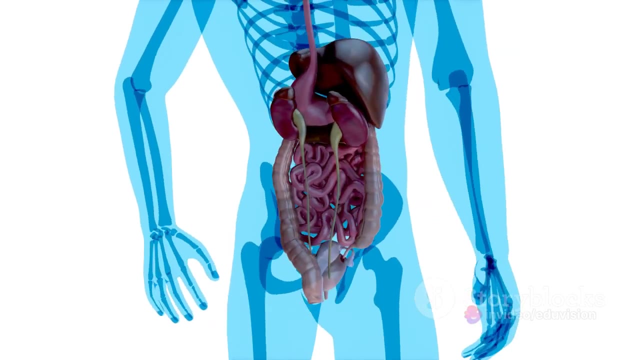 One of the key areas of exploration is the potential link between gut and the enigma of dark matter. If successful, gut could offer a comprehensive explanation for this mysterious substance that makes up about a quarter of our universe. Moreover, the successful establishment of a grand unified theory could revolutionize. 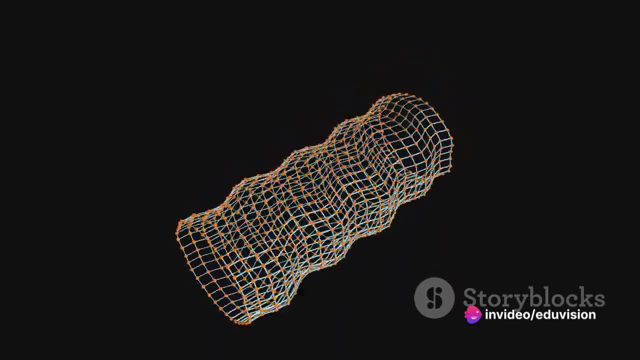 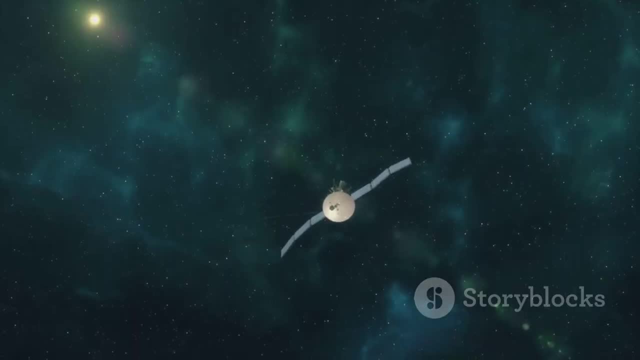 our understanding of the universe. It could provide a unified framework to explain how the fundamental forces of nature interact, a question that has puzzled scientists for centuries. The search for the grand unified theory continues, and the end of this journey could reveal the secrets of the universe. 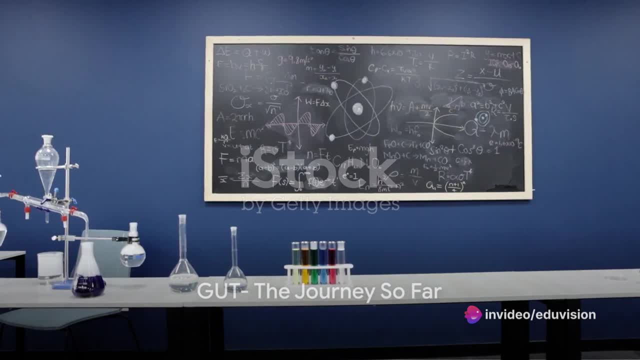 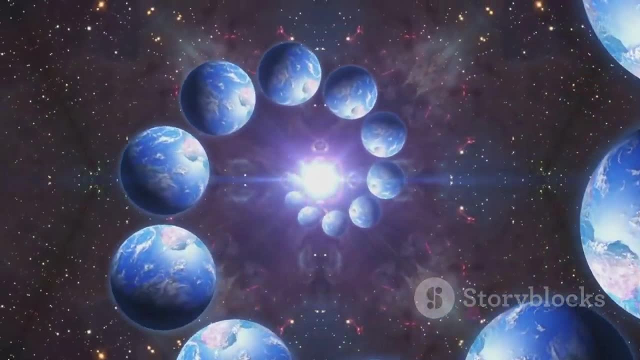 The grand unified theory, a dream of physicists, is a tale of perseverance, innovation and the quest for understanding. It began with a spark, an idea to unify the fundamental forces of nature into a single elegant theory. The road has been riddled. 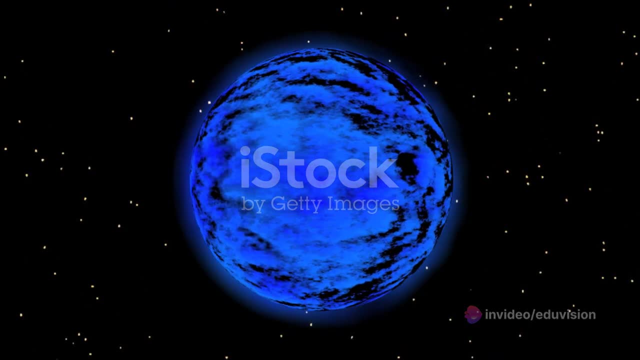 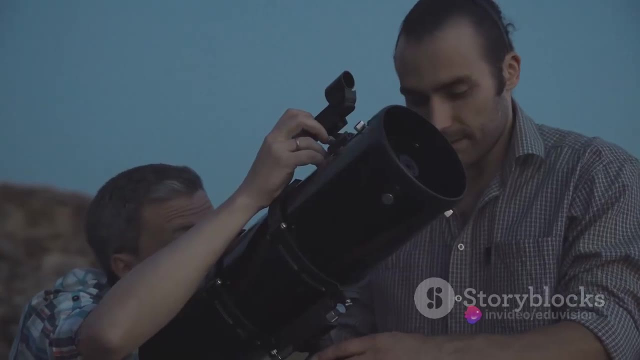 Yet each obstacle has only fueled the flame of scientific curiosity. We've seen breakthroughs that turned the tide, breakthroughs that nudged us closer to the elusive goal. Today, we stand at an exciting juncture. The current state of gut, though not fully realized, is a testament to years of relentless 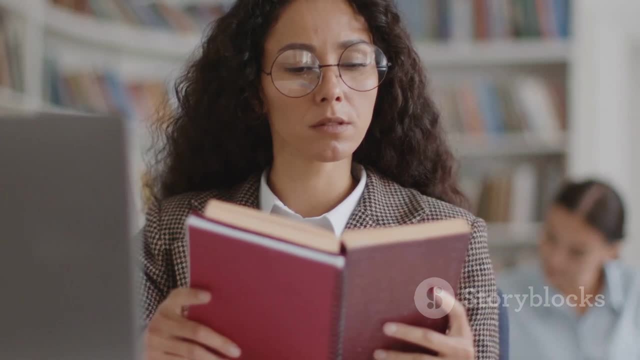 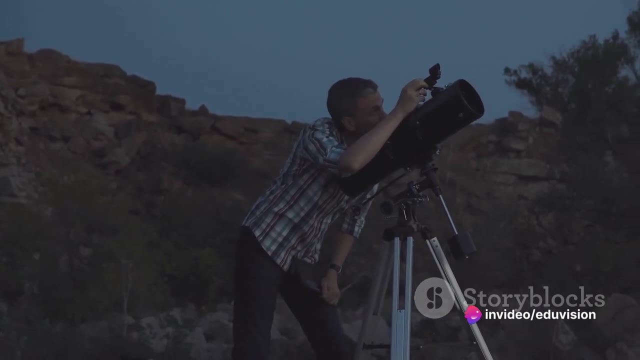 pursuit. It's a story of the human spirit, of our insatiable hunger for knowledge. And in this journey we've not just attempted to unify the forces, but to unify ourselves with the universe, to understand our place within it. As we move forward, we'll be able to see the future of the universe. 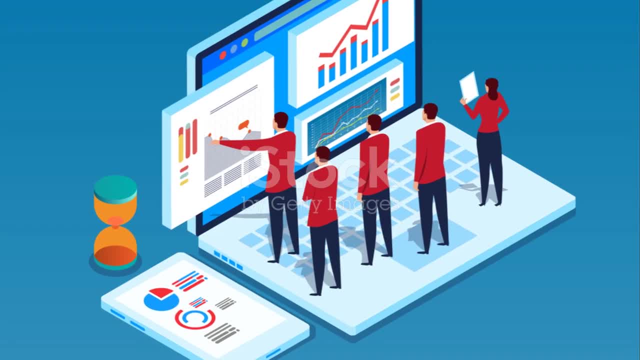 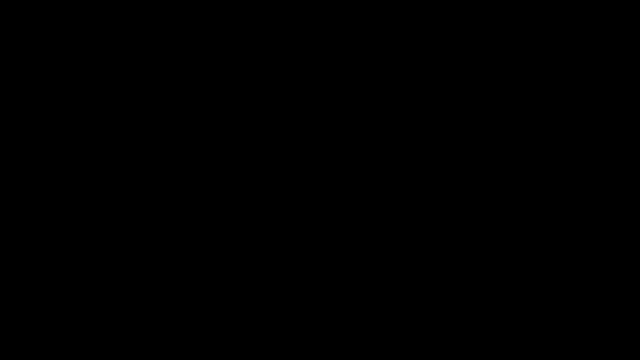 As we inch closer to unifying the fundamental forces, we are unraveling the mysteries that the universe holds. The journey continues and the future of physics is exciting and promising.